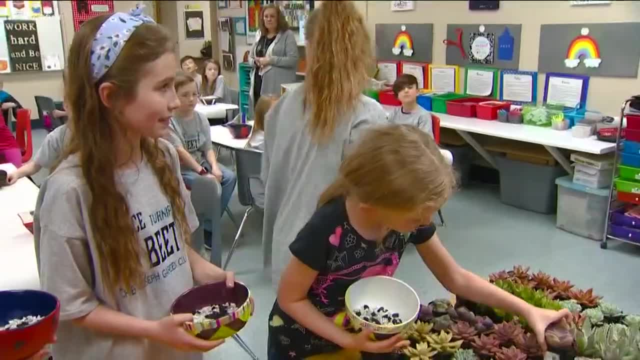 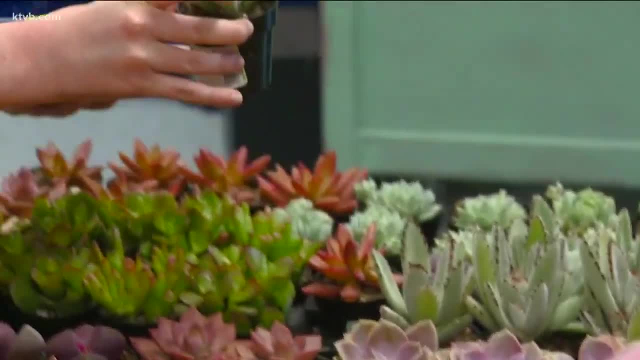 If you accidentally water them too much, this will kind of help so that it can sit there and drain a little bit, because you don't want to overwater your succulents. Then they each select a couple of succulents for their planters. 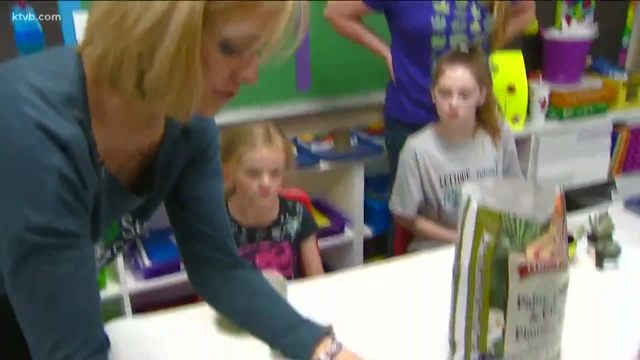 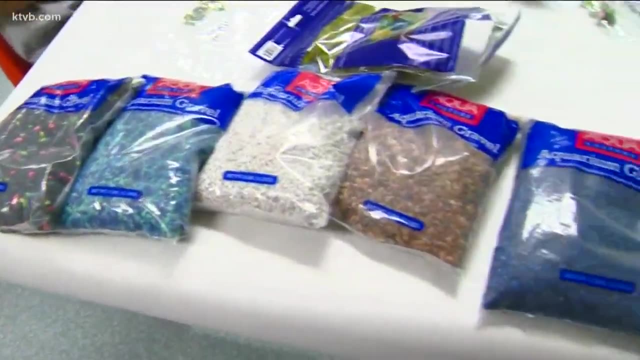 Echeveria, jade plants, aloe vera and others. After a few tips on how to design and plant their containers, the planting and the fun begins, And with some decorative rocks and figurines, the kids' own creativity and imaginations begin to run wild. 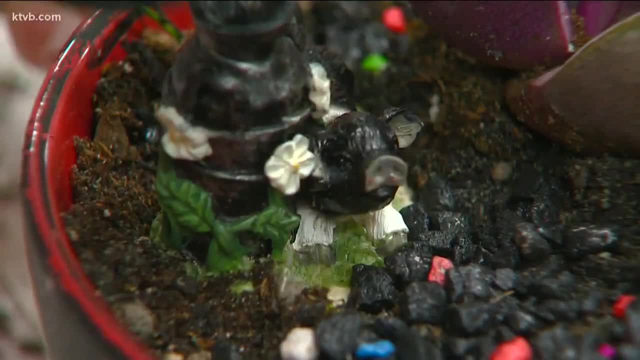 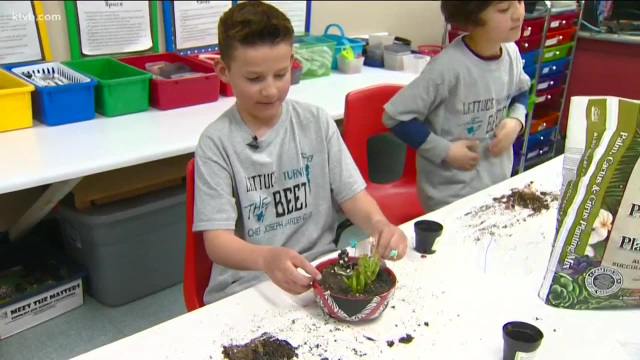 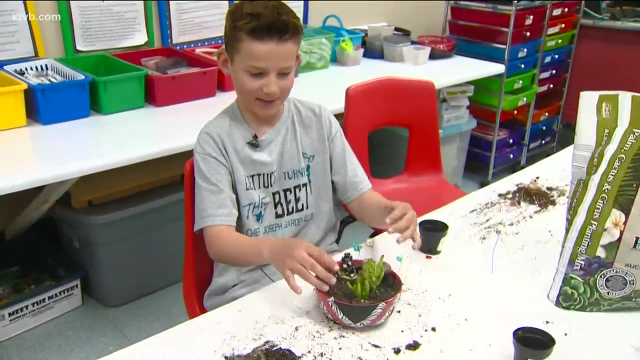 This is my pig that I chose to put in my succulent. It looked like the pig was laying down in the sand And then the flowers can be like the pig's in a meadow or something, And then he's in a different land where there's weird plants and stuff. 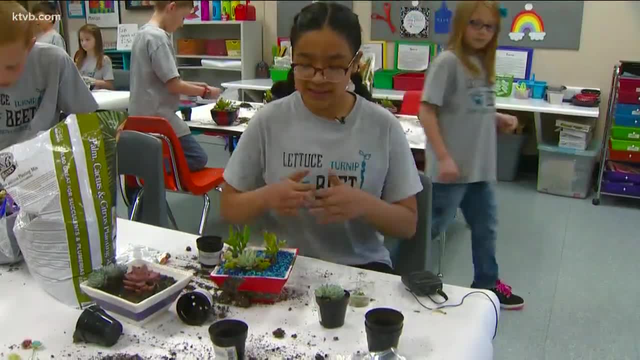 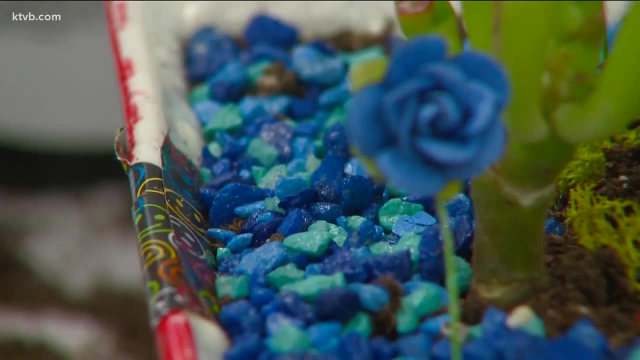 I was thinking. since I love the nature, I just was thinking: a big pond around with lots of rocks on it. After all, blue is Heidi's favorite color and she even nestled a little deer among the plants, And being part of the Garden Club is important to her. 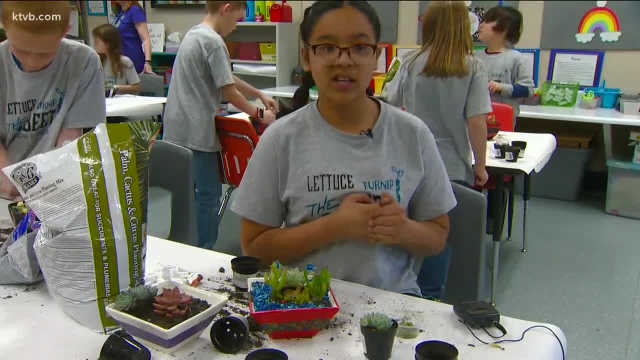 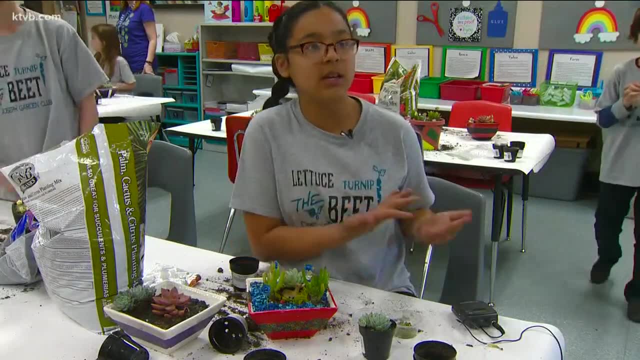 For me. I just think it's very important because it can let kids learn more about plants and how to plant them, because some kids don't know how to plant and they can just plant some. This is a great group of kids We have anywhere from second grade to fifth grade. 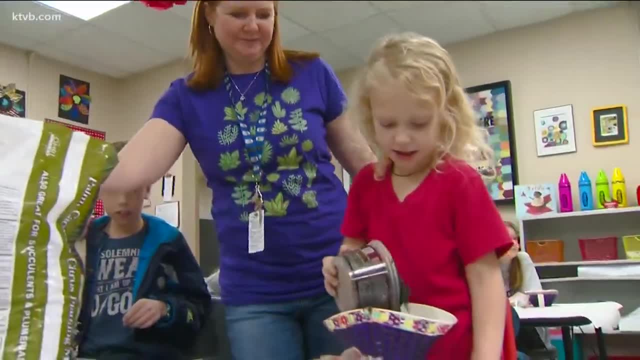 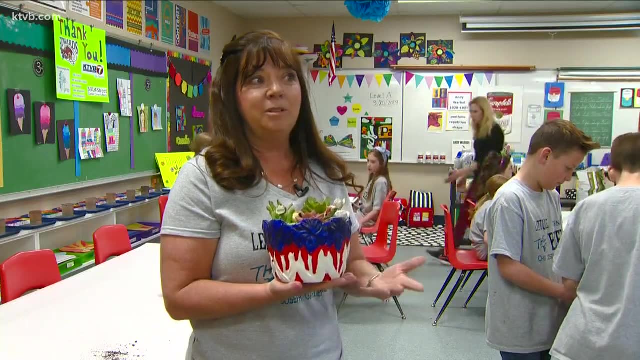 Each year they have to apply to join it, They have to write an essay as to why they should be in the Garden Club, And then they decide what we're going to put in the garden, And during the summer, we donate some of the vegetables to the food bank. 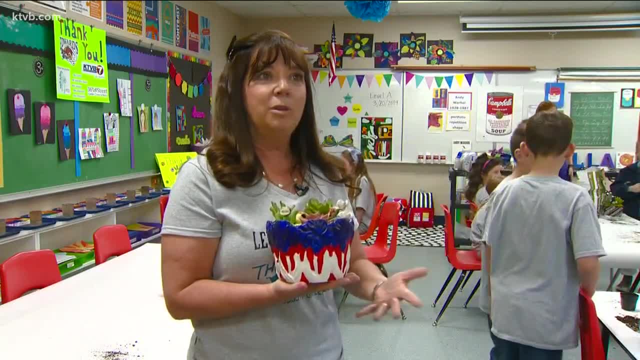 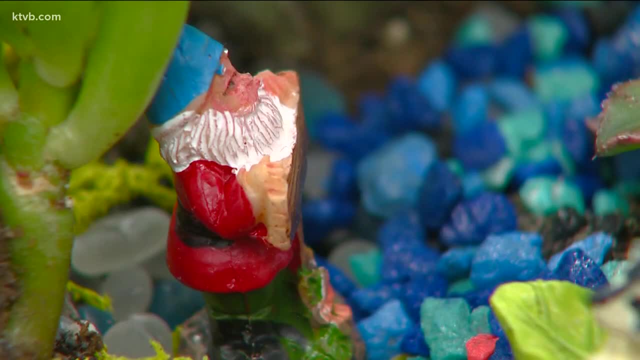 So it kind of shows them the importance of growing the food and sharing with everybody, And the final creations are really living works of art, from the containers to the plants, to the design and decorating, Sharing and working together. these kids have also learned another important thing about gardening. 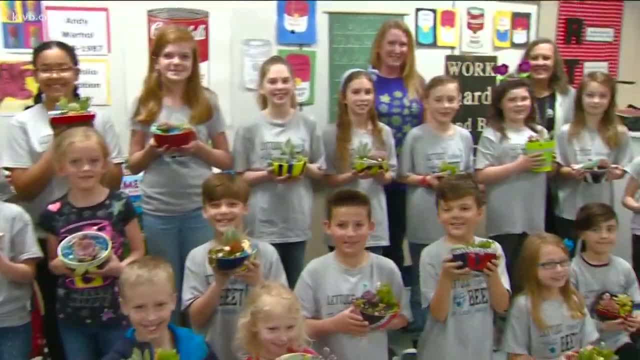 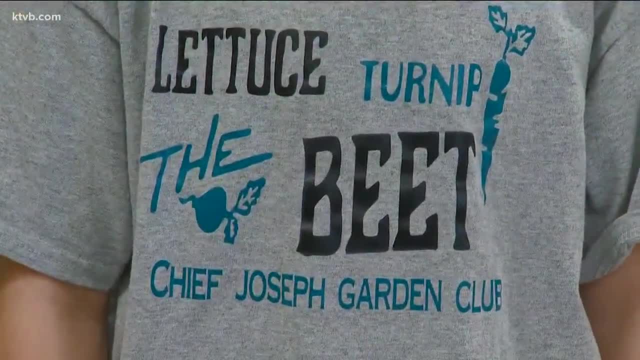 You can grow it, And so can you just like the Garden Club here at Chief Joe's Garden. It's the Joseph Elementary School For Idaho's News Channel 7, and You Can Grow It. I'm Jim Duthie. I'm so glad they finally zoomed in on the shirt, because I'm like: what does their shirt say?